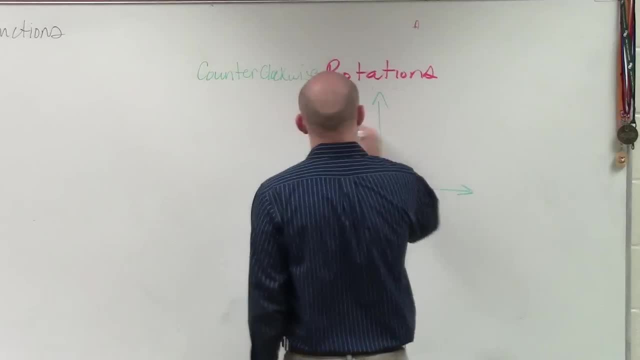 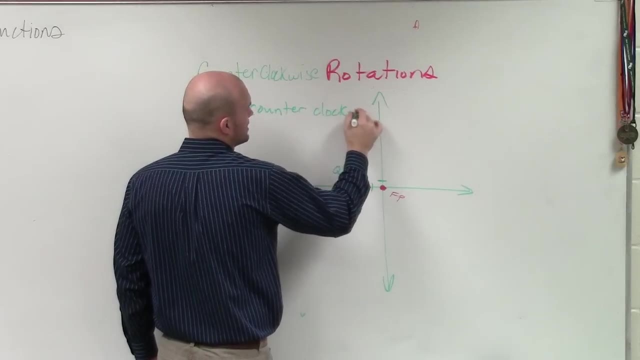 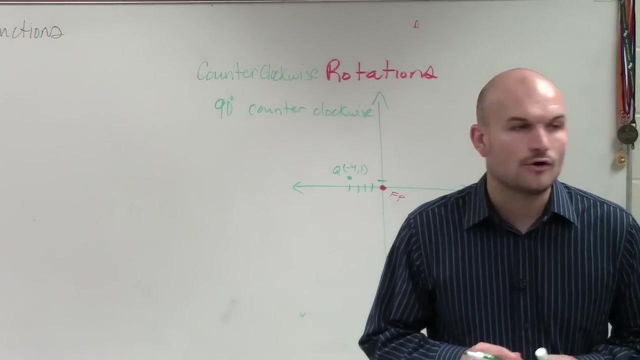 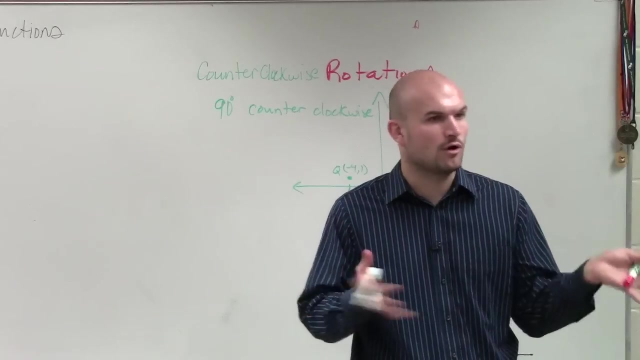 How are we going to rotate this 90 degrees? So let's say 90 degrees counterclockwise. So what is going to be the formula for us to be able to rotate something counterclockwise 90 degrees? Well, remember reflections, guys. I had x and y, Then I told you how to do what. 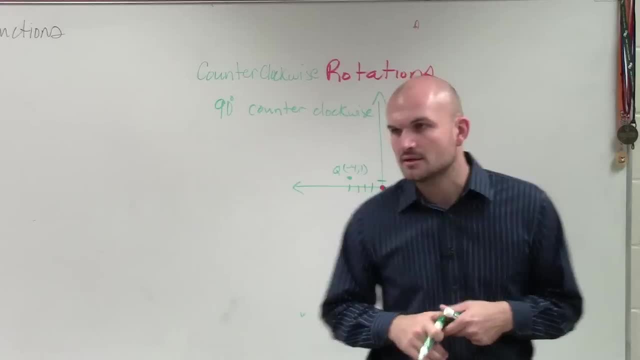 was negative, for which one, or when to swap them. Do you guys remember doing that? So for rotation, we're going to do negative 1,, 2,, 3, 4, negative 1,, all right. And then for rotations, this is the exact same thing. When you want to do a 90 degree rotation, 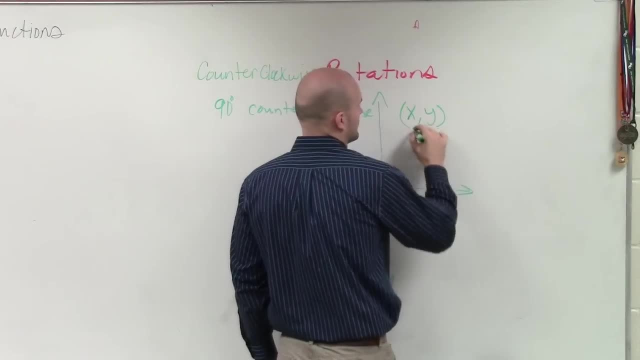 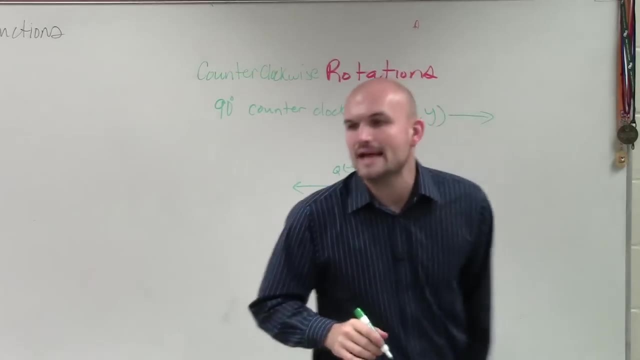 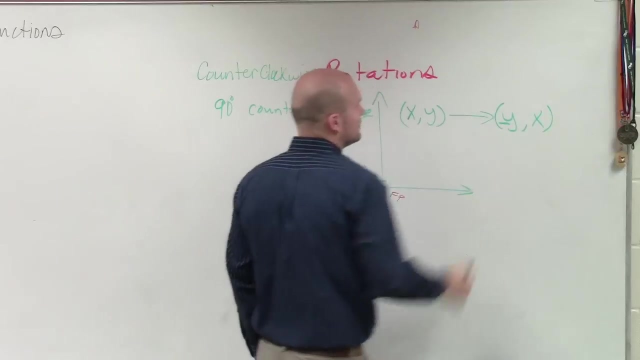 if I have a coordinate, point x, comma y, and I want to rotate it 90 degrees. now what I'm going to do, Mario, is swap the variables and then make the y coordinate negative. So, Mario, that's going to be really important for you to be able to write down, for that. 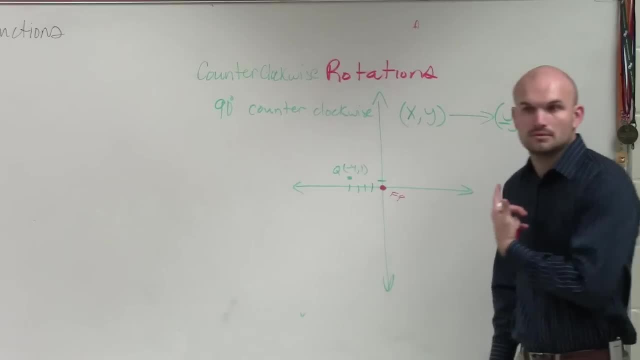 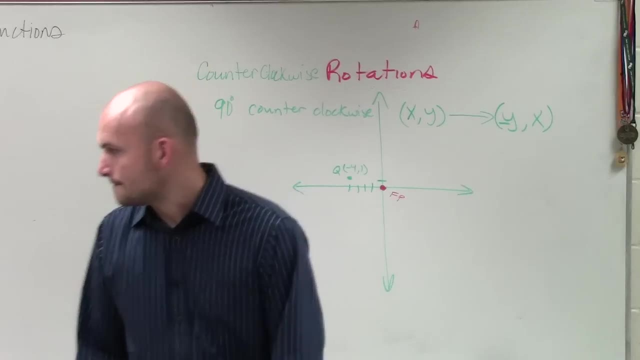 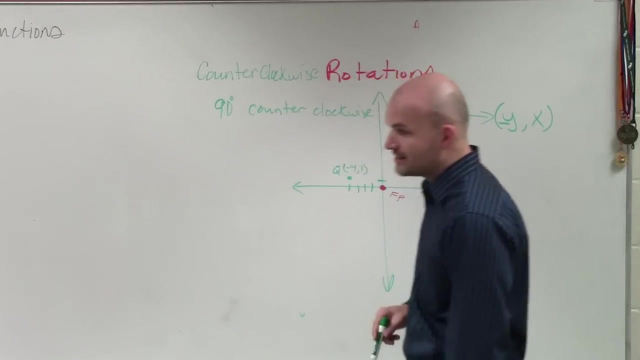 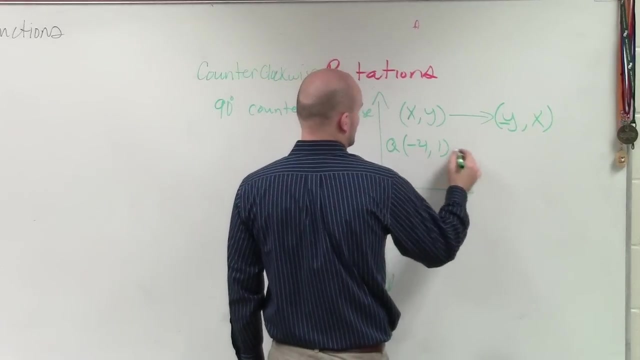 okay, Mario, You need to have that written down. Okay, Yes, Why is the y a negative now? Well, let's go and take a look at what this point would look like. okay, So let's go and try this to our point q. So q we have is negative 4, 1.. If I go ahead and find q prime, 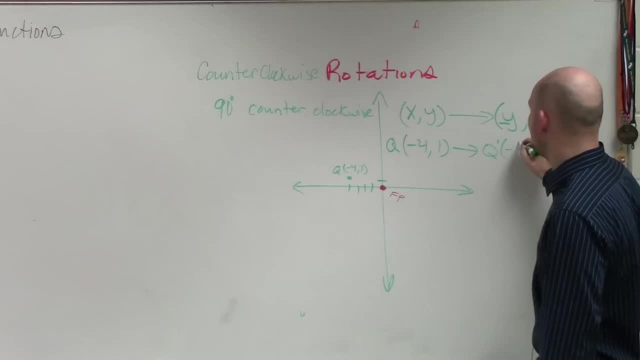 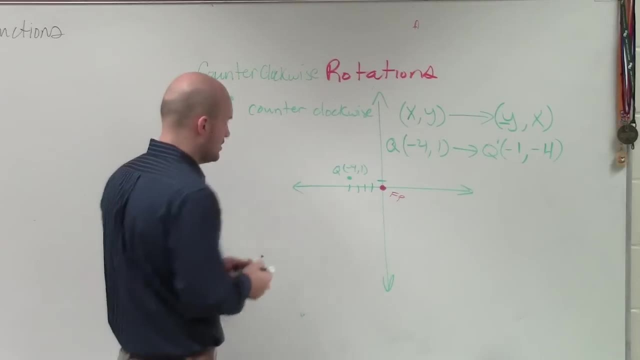 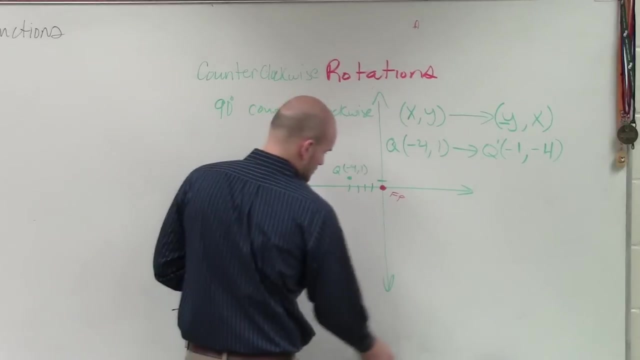 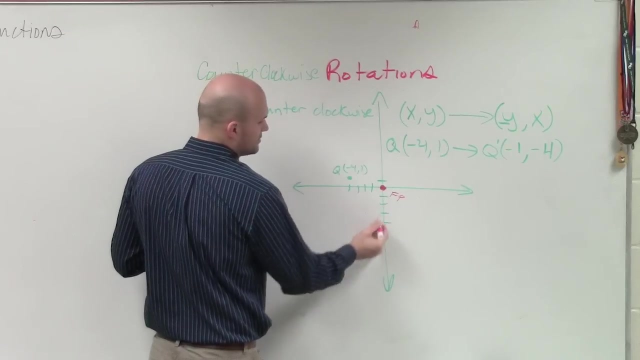 by following this rule, I now swap this to negative 1, comma, negative 1.. So what's the y Negative 4.. So let's go ahead and take Camila. what this new point would look like, I'm sorry, Okay. So now it's at negative 1, 1,, 2,, 3,, 4.. So negative 1, down 4.. That's going to be. 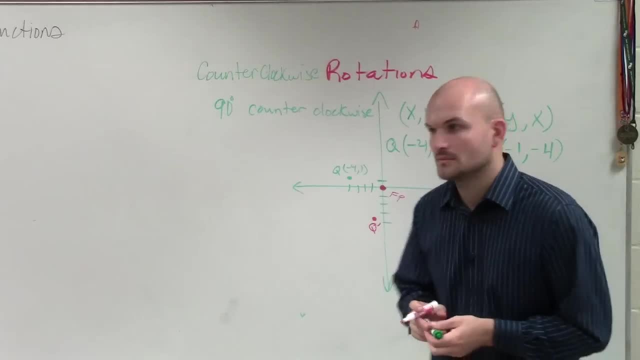 what a 90 degree rotation looks like. all right, And think about it. If you guys took this and you rotated, you're going to get negative 4, 1, 2, 3, 4.. That's going to be what a 90 degree rotation. 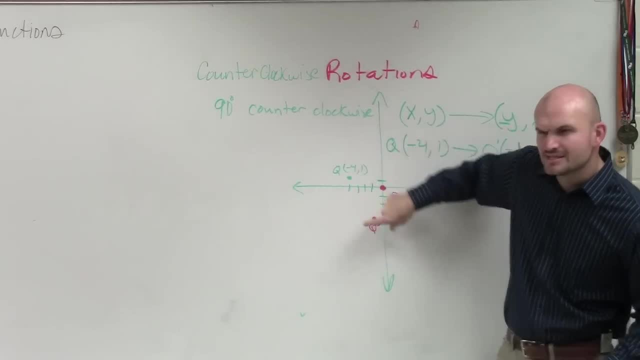 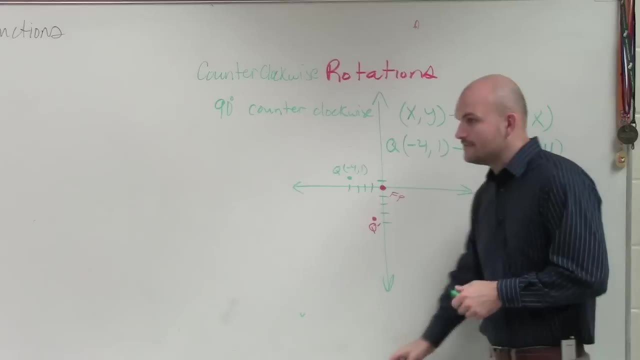 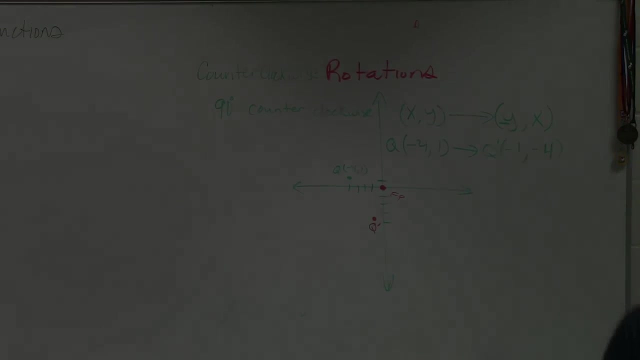 looks like. all right, And think about it. If you guys took this and you rotated to a 90 degree, you rotate this point 90 degrees, does that look like where that point should land? Yes, Yeah, exactly Right. And if you guys want me to show you a trick, OK.